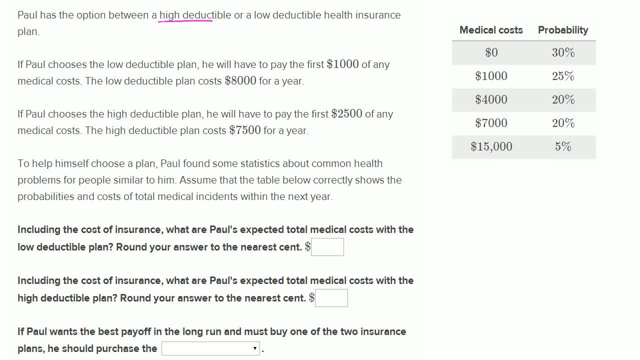 Paul has the option between a high deductible or a low deductible health insurance plan And when we talk about the deductible and health insurance, if someone says that they have a plan with a $1,000 deductible, that means that the insurance company only pays the medical costs after the first $1,000. 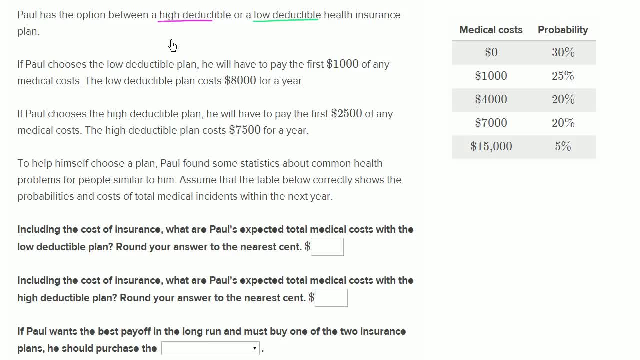 So if you have a $1,000 deductible and you say incur medical costs of $800, you're going to pay that $800. The insurance company won't pay anything If you have a deductible of $1,000 and your total medical costs are $1,200,. 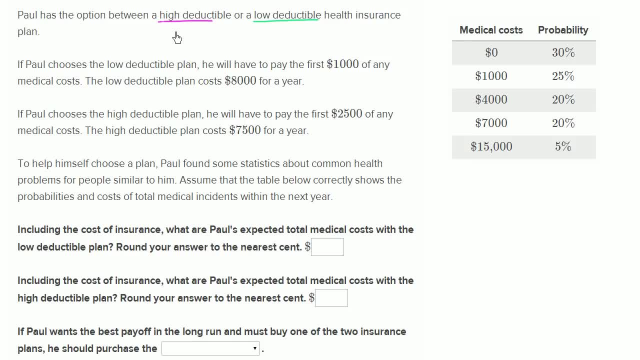 you're going to pay the first $1,000 and then the insurance company will kick in after that. So with that out of the way, let's think about his two plans. If Paul chooses the low deductible plan, he will have to pay the first $1,000 of any. 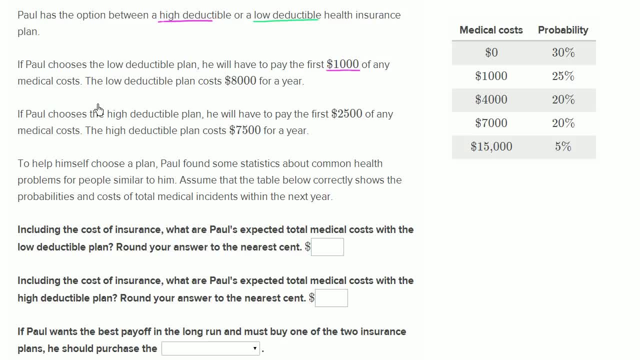 let me do that in purple: the first $1,000 of any medical costs. The low deductible plan costs $8,000 for a year. So in this situation he's going to pay $8,000 to get the insurance If he has $900 of medical expenses. 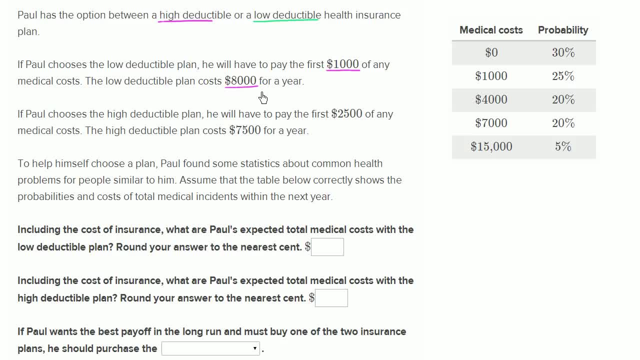 the insurance company still pays nothing. If he has $2,000 of medical expenses, then he pays the first $1,000 and then the insurance company would pay the next $1,000.. If he has $10,000 in medical expenses, 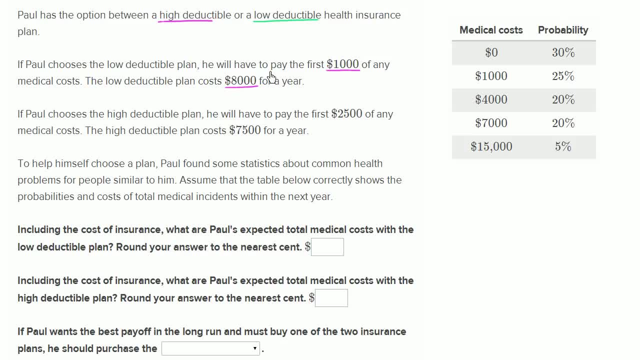 he would pay the first $1,000 and then the insurance company would pay the next $9,000.. If Paul chooses a high deductible plan, he will have to pay the first $2,500 of any medical costs. The high deductible plan costs $7,500 a year. 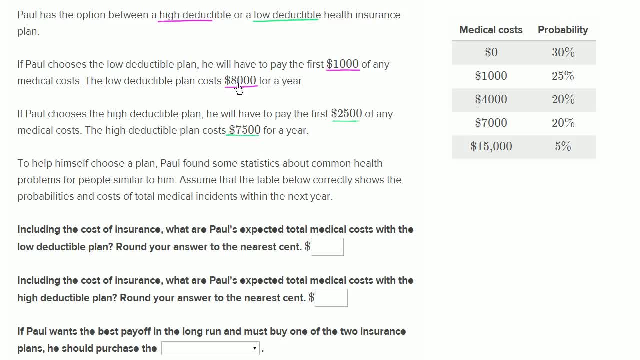 And it makes sense. It makes sense that the high deductible plan costs less than the low deductible plan because here the insurance doesn't kick in until he has over $2,500 of medical expenses, while here it was only $1,000.. To help himself choose a plan. 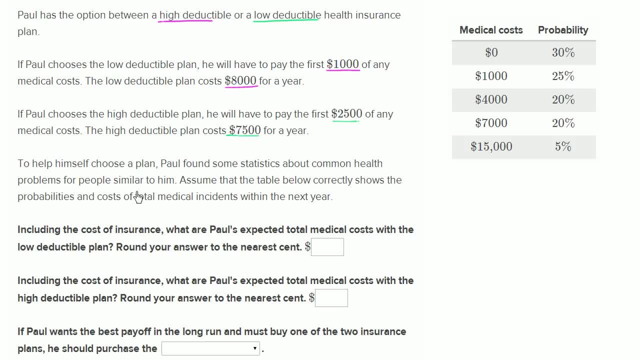 Paul found some statistics about common health problems for people similar to him. Assume that the table below- and I put it up here on the right- correctly shows the probabilities and costs of total medical incidents within the next year. So this right over here it's saying: 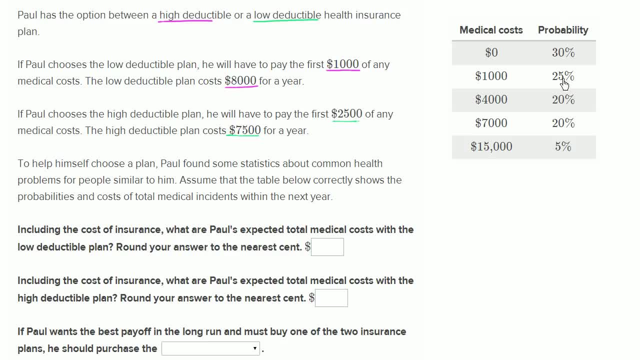 what's the probability he has zero in medical costs. What's the probability he has a 25% probability of $1,000, 20% probability: $4,000.. And this is a simplification, a pretty dramatic simplification from the real world. 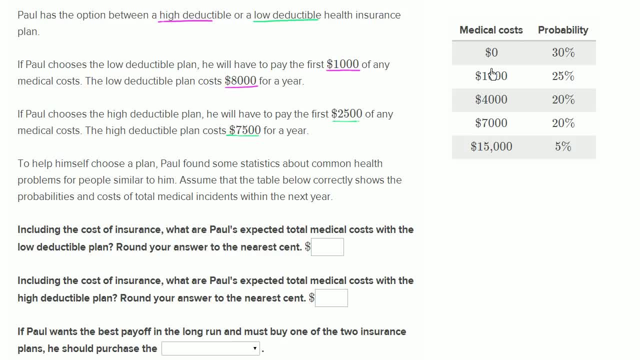 In the real world, the way this makes it sound is there's only five possible medical costs that someone might have: zero: 1,000, 4,000,, 7,000, and 15,000.. In the real world, you could have $20 in medical costs. 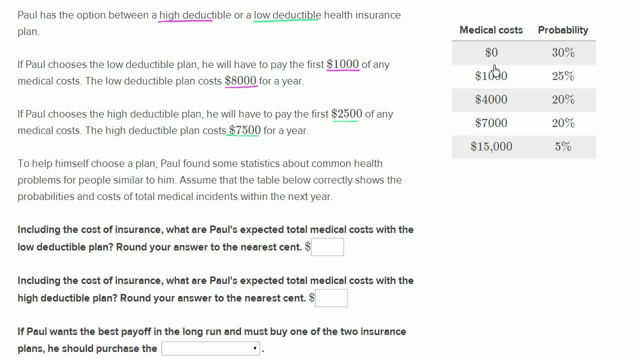 You could have 20,000.. You could have $999.. So in the real world there's many, many more situations here that you would have to kind of redistribute the probabilities accordingly. But with that said, this isn't a bad approximation. 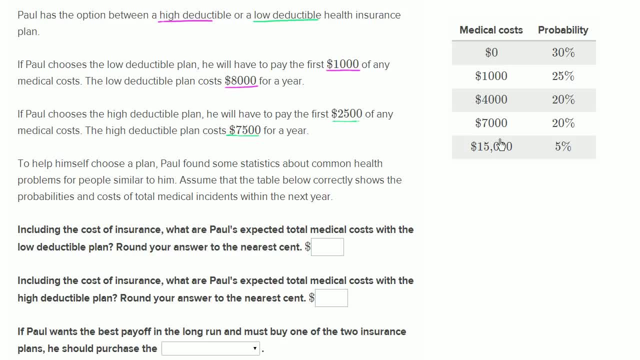 It's just saying: okay, you know roughly if you wanted to construct this, so it's easier to do the math which the problem writers have done. say: look okay, 30%, zero, 25%, $1,000.. 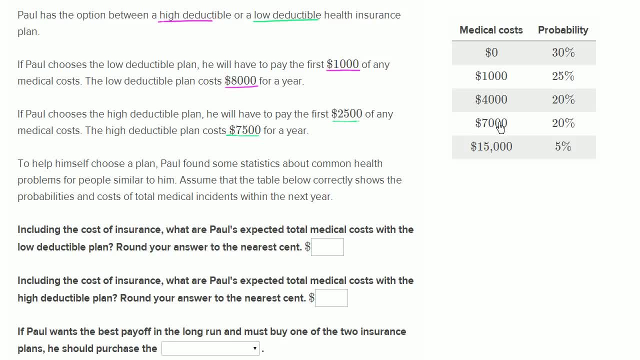 This is pretty indicative If you had to kind of group all of the possible costs into some major, major bucket. So it's probably at least a pretty good method for figuring out which insurance policy someone should use. So they say including the cost of insurance. 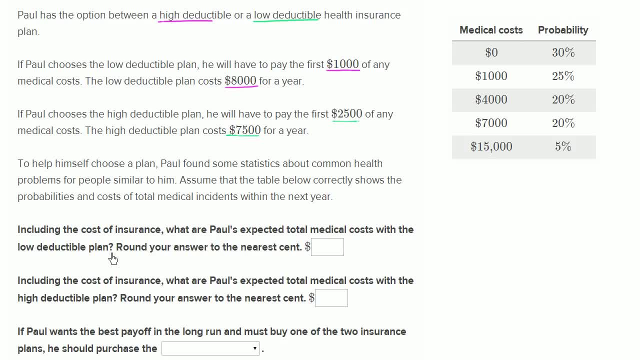 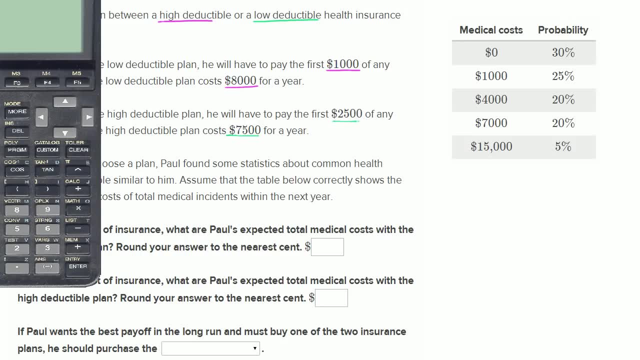 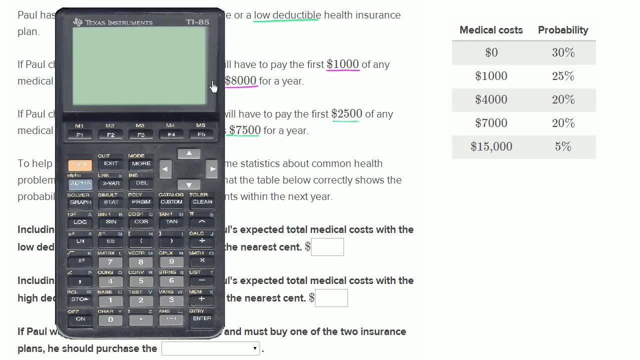 what are Paul's expected total medical costs with the low deductible plan? Round your answer to the nearest cent. So actually I'll get the calculator out for this. So at the low whoops with the low deductible plan here low deductible plan he's going to have to spend. 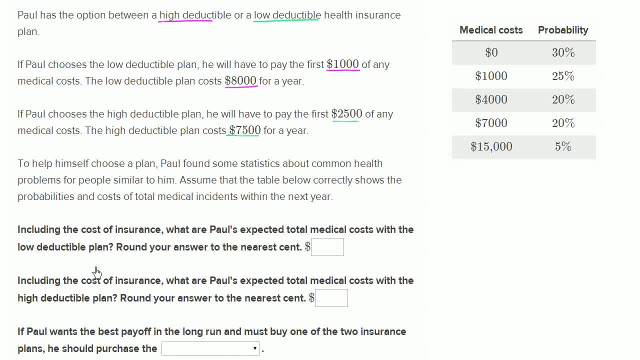 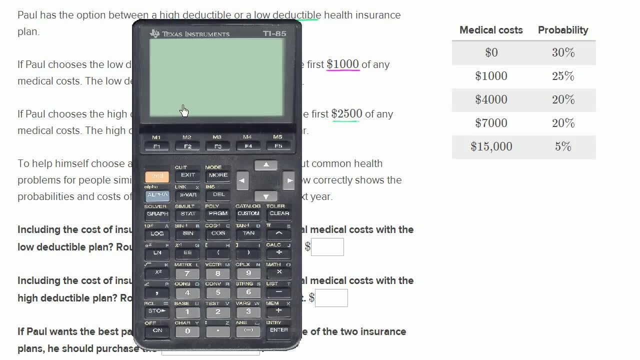 the total cost. he's going to spend $8,000, no matter what- Whoops, what happened to my calculator? He's going to spend $8,000.. My God, I'm having issues. He's going to spend $8,000, no matter what. 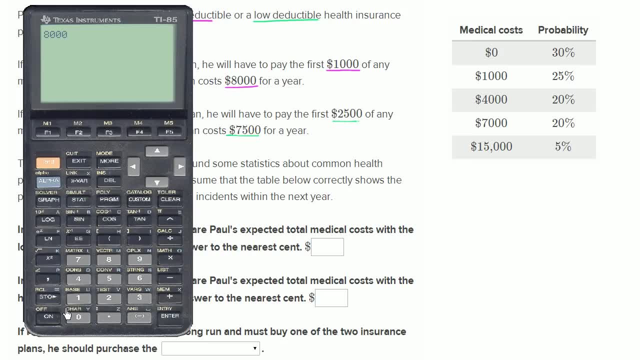 So that is $8,000.. And then let's see, There's a 30% probability he spends nothing. I could just write that as plus .3 times zero And I will write it just so that you see I'm taking that into account. 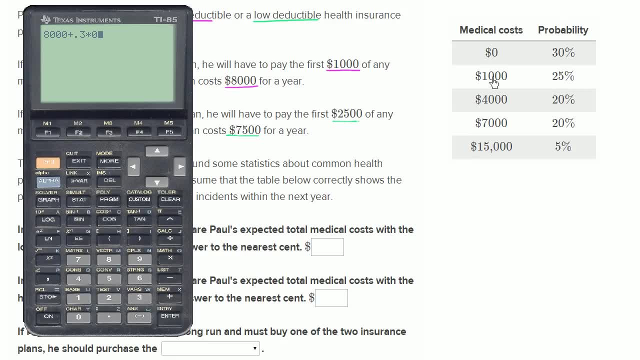 And there's a 25% chance that he has $1,000 in medical costs And in the low deductible plan he still has to pay that $1,000.. So plus .25% chance that he pays $1,000.. 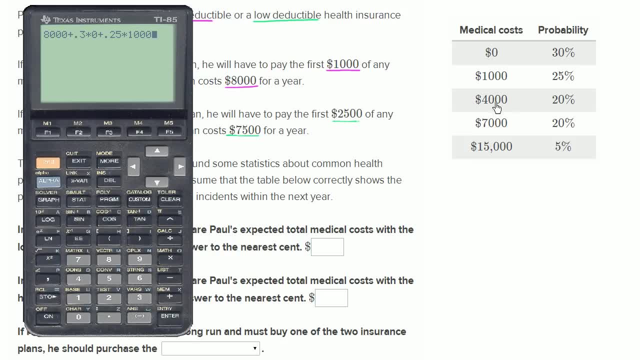 And then you might say, okay, plus .2 times 4,000.. But remember, if his medical costs are 4,000, he's not going to pay that 4,000.. He's only going to pay the first 1,000.. 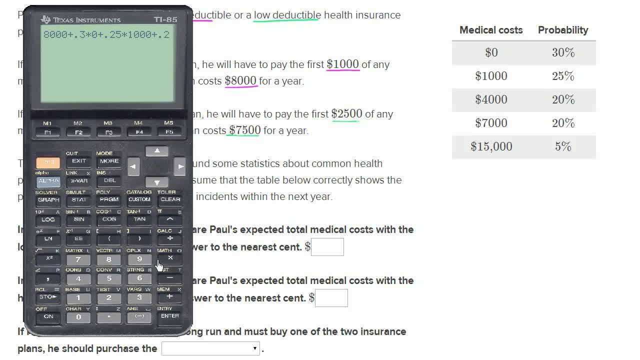 So it's really plus .2.. In this situation, his out-of-pocket costs are only $1,000.. The insurance company will pay the next 3,000.. So .2 times 1,000.. And then plus .2, 20% chance. 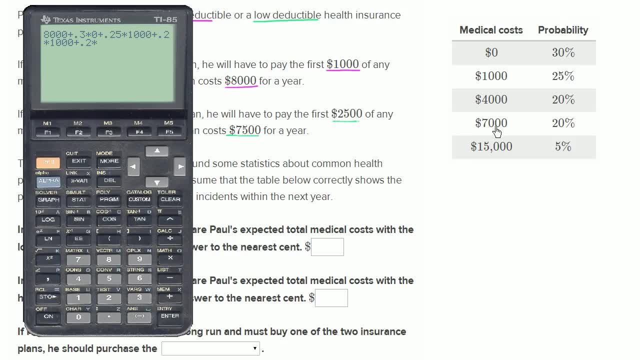 Even if he has 7,000 in medical costs, he's only going to have to pay the first 1,000.. So .2 times 1,000.. 1,000 again, And then plus .05 times, once again 1,000.. 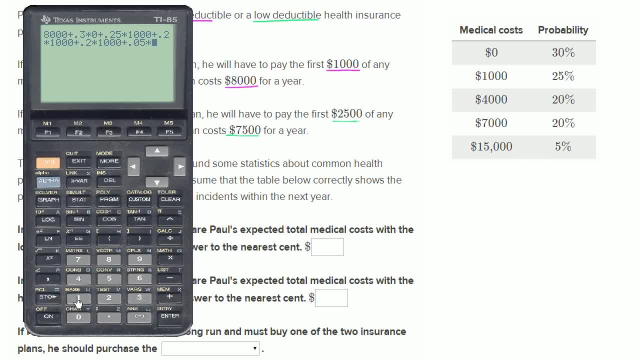 If he has 15,000 in expenses, he's only going to have to pay the first 1,000.. Times 1,000. And we get $8,700.. And one way you could have thought about it is: OK, he's going to have to pay $8,000, no matter what. 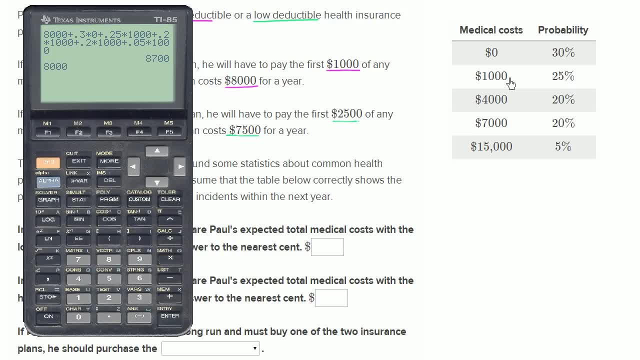 And all of the situations where he ends up paying, that's anything. That's These four situations right over here. There's a 70% probability of falling into one of these four situations And in any one of these he only has to pay $1,000. 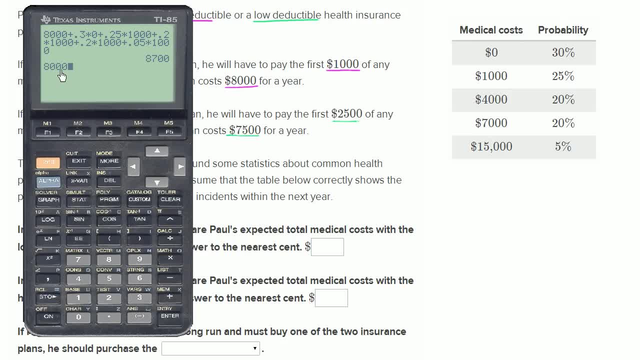 The insurance company pays everything after that. So you could say 8,000 plus there's a 70% chance that he's going to pay 1,000.. And once again, this table is a pretty big simplification from the real world. 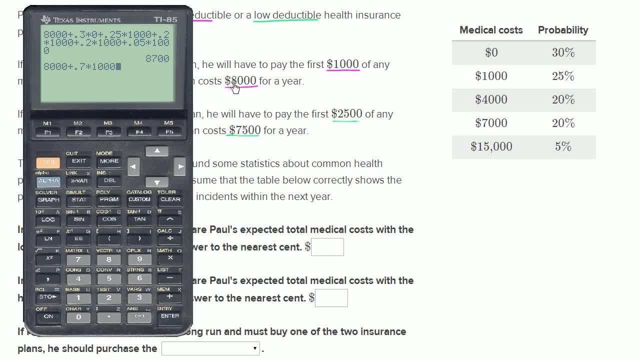 There's probably a lot of scenarios where he would have to pay $500 or $600 or whatever it might be, But let's just go with this And so that's essentially a simplification. There's a 70% chance that he's going to have to pay $1,000. 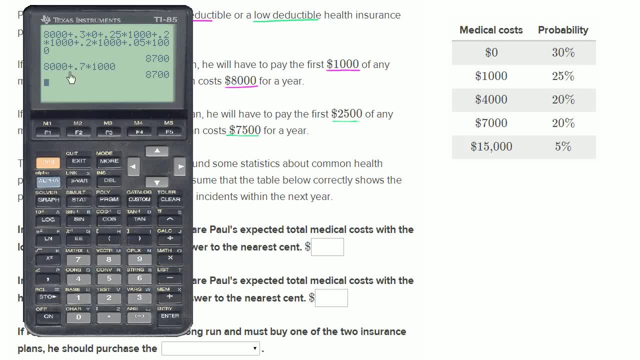 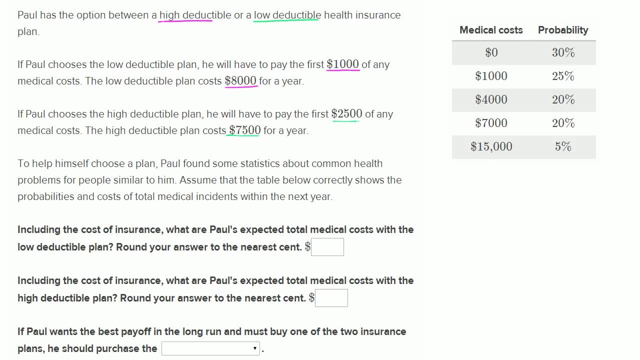 And so that's the $700 expected cost. from that, plus the 8,000 from the insurance, gets us to $8,700.. So let's write that down: So $8,700.. My pen is really acting up. I don't know what's going on here. 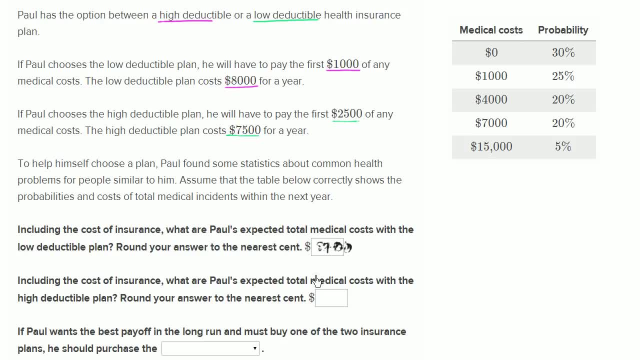 I think I have to get a new tablet 80. You can't even read that. Let me write this: $8,700. Including the cost of insurance, what are Paul's expected total medical costs with the high deductible plan? Round your answer to the nearest cent. 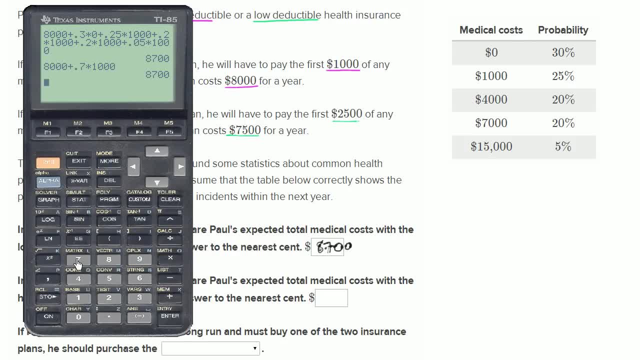 So let's look at the high deductible plan. So he's going to pay $7,500, no matter what, And then So we could write $0 times 30% or 30% times $0.. But that's just going to be 0.. 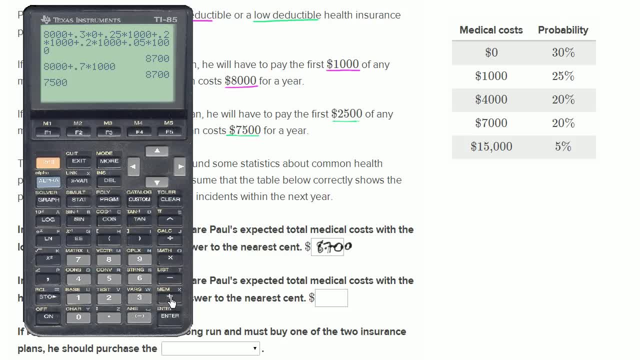 There's a 25% chance he spends $1,000.. So plus 0.25 times $1,000.. There's a 20% chance plus 0.2.. He's not going to spend $4,000 here. 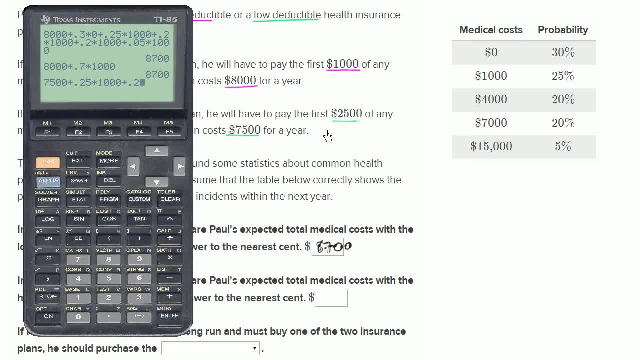 He's going to have to spend the first $2,500. So it's a 20% chance he spends $2,500.. OK, So times $2,500.. Insurance company will pay the next $1,500.. Plus another 20% chance. 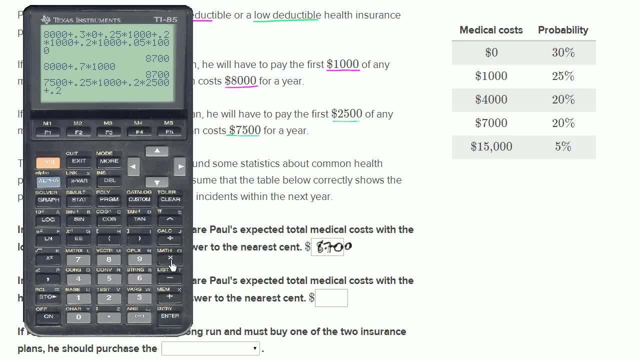 Even in this situation, he only has to pay $2,500.. So times $2,500.. And then finally, plus, there's a 5% chance. Even in this situation, he only has to pay the first $2,500. 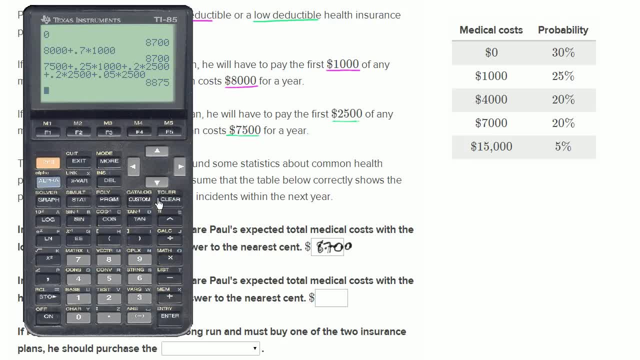 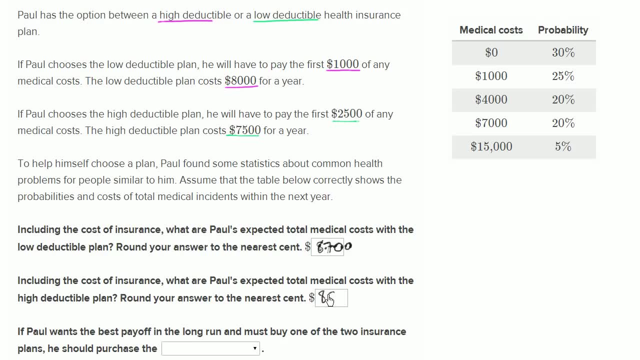 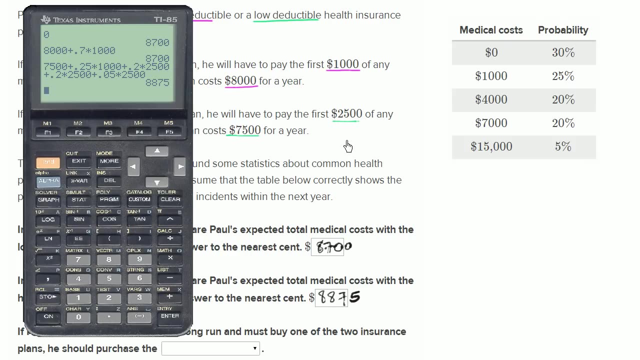 Times, $2,500 gets us to $8,875.. OK, That's good. OK, $8,875.. So $8,875.. And once again, you could think about it as OK, there's a 25% chance that he pays $1,000. 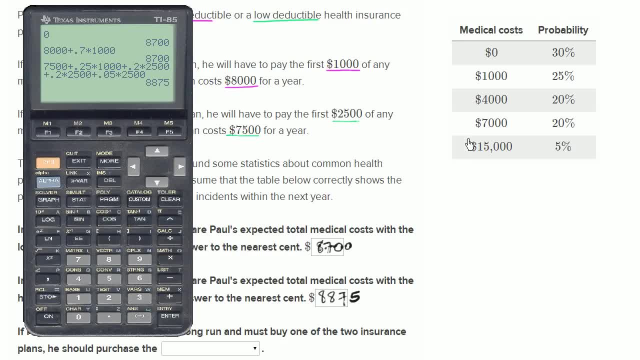 And then there is a 45% chance that he pays $2,500.. All of these situations he's paying $2,500. But either way you would get $8,875.. If Paul wants the best payoff in the long run and must buy one.